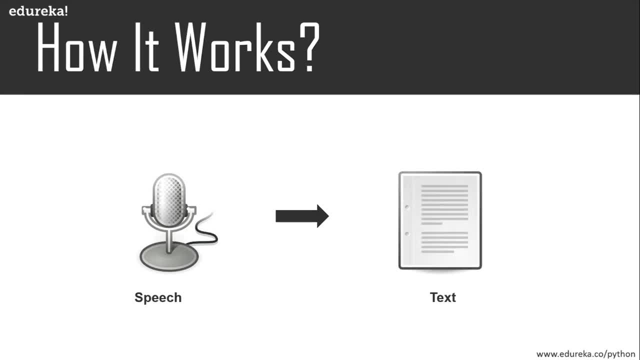 the spoken utterances to text. There are various real-life examples of speech recognition systems. For example, we have Siri, which will recognize the speech and translate it into text. Now the real focus is: why do we actually need a speech recognition system? The main reason is speech is actually the most common means. 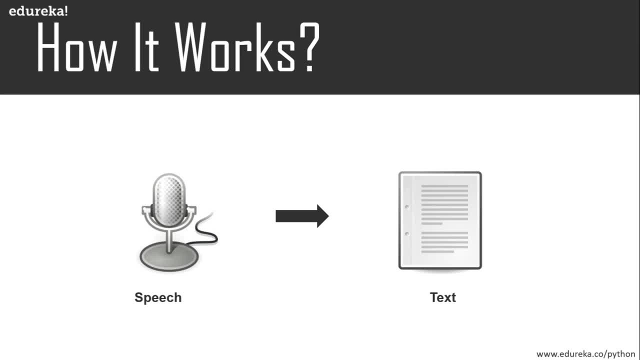 of communication. majority of the population in the world relies on speech to communicate with one another. the advantage of speech recognition system overcomes the barrier of literacy as well. It will serve both the literate and the illiterate as it is focused on the spoken utterances. 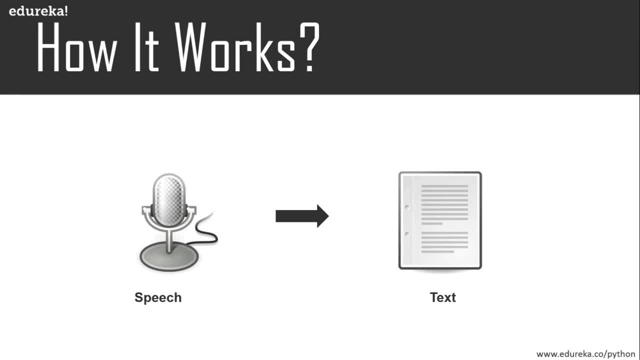 and in this way we can even make a safe inventory of the endangered languages around the world. So now that we know how speech recognition works and serves us in real time, Let's take a look at the challenges that are faced by any speech recognition system. 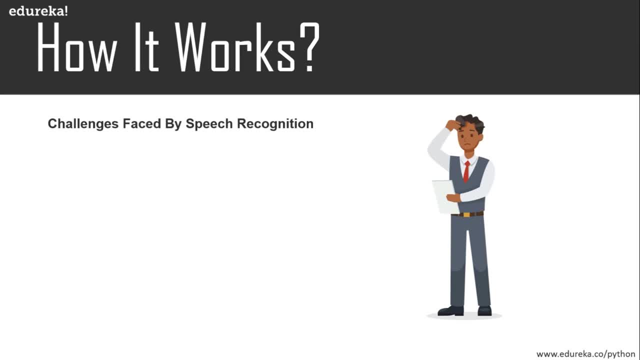 a speech recognition system becomes difficult to make because we have so many sources of variability. For example, different person may have a different style of speaking or may have an accent as well. For example, we have American accent, We have British English, American English and there are so many more actions when we are talking, 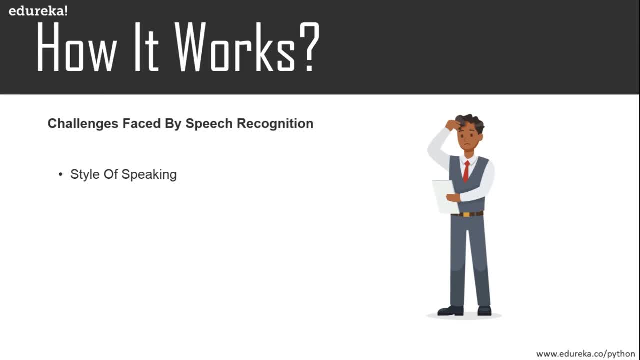 about different style of speaking. pronunciation also makes it difficult for any speech recognition system to translate the speech altogether. Then we have different environment as well. For example, an isolated room and an auditorium will have different background noises. I think this goes without saying that echo also can contribute. 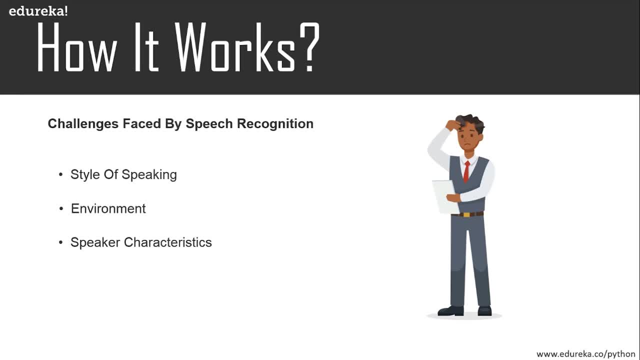 to a lot of noise as well. moving further, the speaker characteristics also differ. For example, an old person's voice compared to that of a child or an infant will have significant variability. and not to mention the language constraints, guys. some spoken utterances may not have a viable meaning. 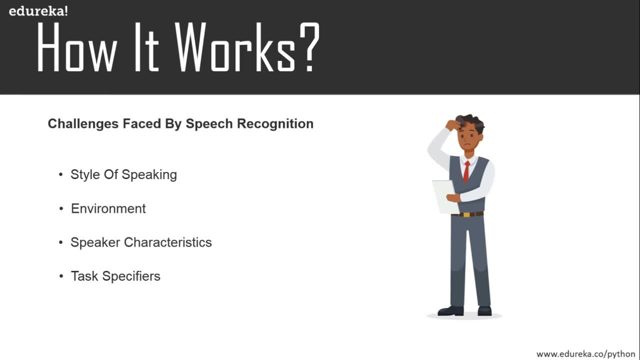 when it comes to translation. So these are the challenges that are faced by any speech recognition system. So now that we know what are the challenges, let's take a look at the journey of speech recognition system from where it started and how far we have come so far. 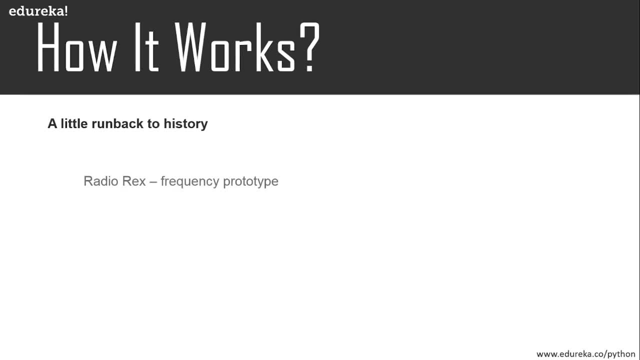 So let's take a little run back to the history, guys. The very first prototype of speech recognition was, in fact, a toy. it came around 1920s, guys, So it had a dog sitting in the doghouse which was connected to a spring and whenever a person used to call. 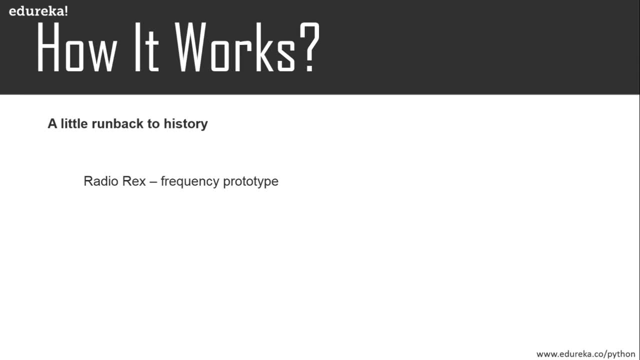 out the name Rex. it used to jump right out of the box. It was a very cool toy to play with, but the problem with the prototype was that the spring was connected to a electromagnet which was sensitive to energies and frequencies around 500 Hertz. 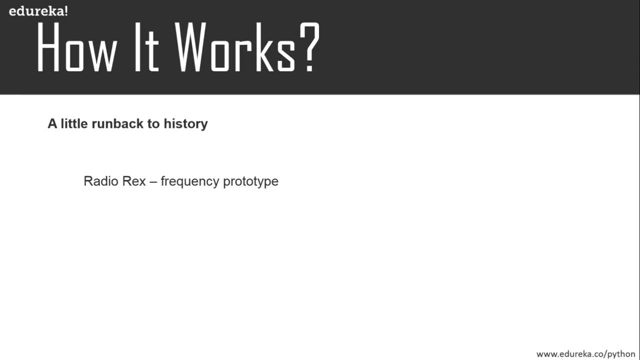 So it was purely a frequency detector but we can say it was remotely working on speech recognition and the major setback was it could only detect the speech from adult men because, we can see, only the adult men could utter the word Rex around that frequency. So the next one is the shoebox which came around 1962. 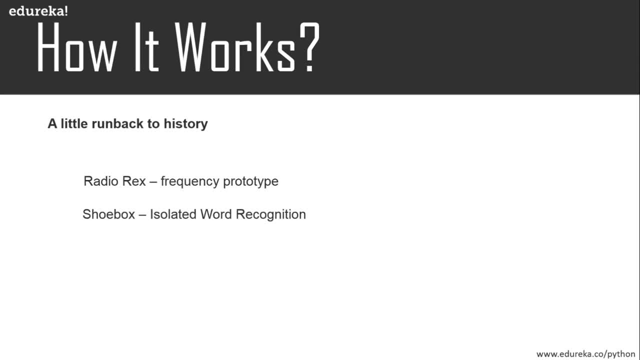 and it was made by IBM. Now this model was able to recognize connected strings of digits and also perform a few arithmetic operations. So in total we had 16 words in the vocabulary. So it was doing isolated word recognition, since you had a lot of pause between the strings. 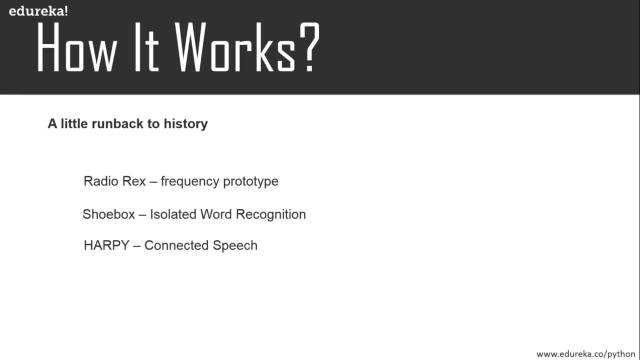 and then came harpy from CMU, which was able to recognize connected strings of speech from a thousand word vocabulary. then around the 1980s, people started using statistical models and one of the machine learning paradigms that was used was hidden Markov models by 2006.. 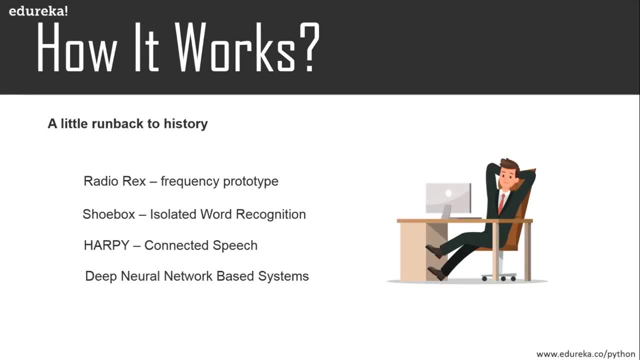 The world was introduced with deep neural networks and since then most of the speech recognition systems are based on deep neural networks, which can use up to 10,000 words library, So the numbers can go higher, of course. So this is all about the history of speech recognition system. 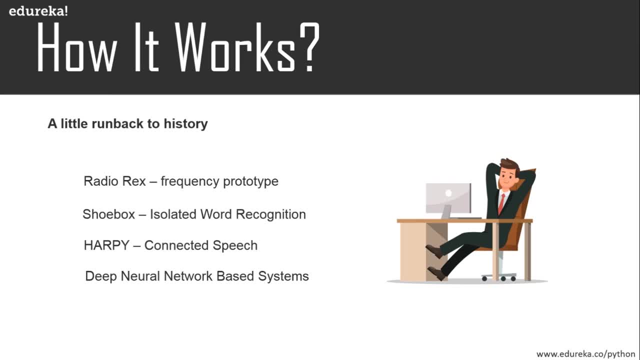 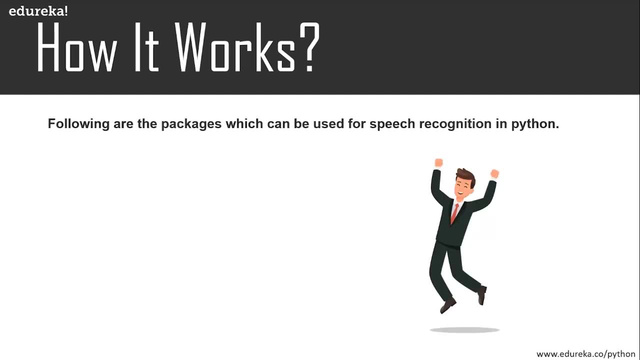 Of course, There were so many other models that people worked on. These are only a very few that I have told you about, guys. So now that we are done with the history as well, Let's take a look at different packages that we can use for speech recognition in Python. 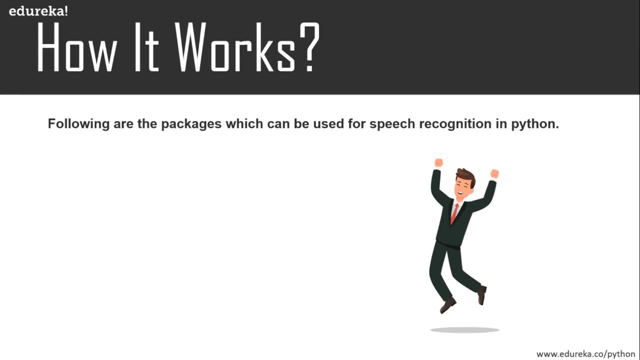 So following are the packages which can be used for speech recognition in Python. So first one is the API AI, then we have assembly AI and then there is Google Cloud speech, Then there is speech recognition which we are going to use in our use case, and I'm going to explain how we are going. 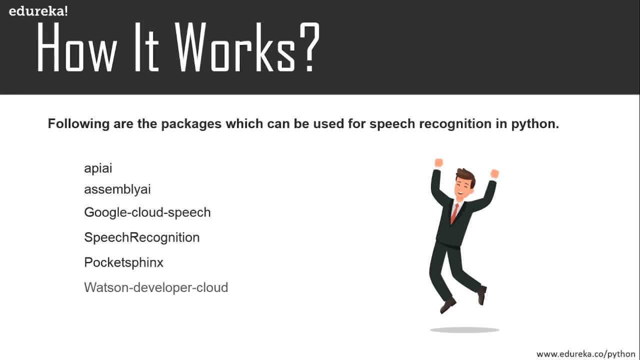 to use the speech recognition module, and then we have pocket Sphinx, Then there is Watson developer cloud and then there is wit as well. So these are the packages which can be used in speech recognition for Python guys. Now let's try to understand how we can install speech recognition. 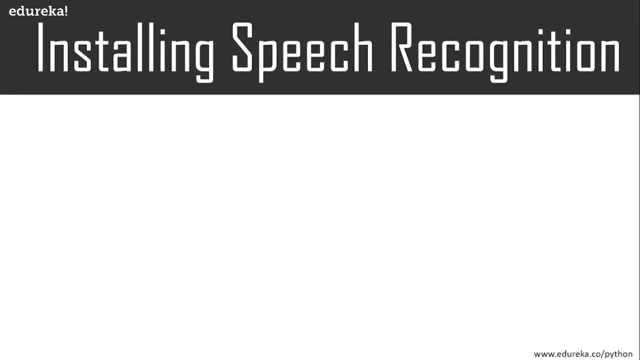 in Python. So I hope this goes without saying, guys. We are going to use this simple statement in our terminal guys, which is pip- install speech recognition. So let me take you to PyCharm guys, where we will install speech recognition. So this is PyCharm guys. 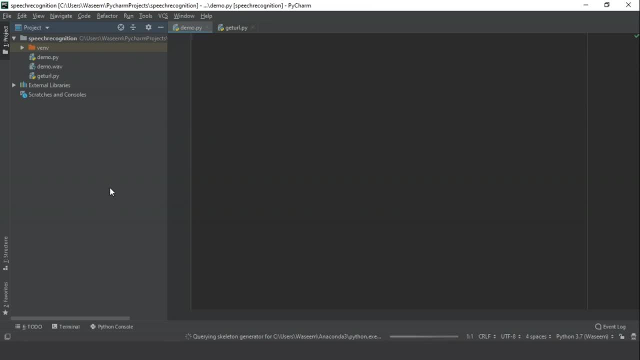 and I have already created a project that I'm going to show you when I'm showing you the use case. guys, So to install speech recognition you have to open the terminal and, inside this, just run this command in spit: install speech recognition, Because I have already installed it. 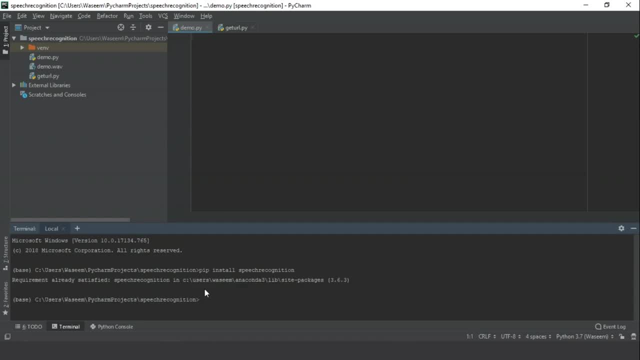 It will show me a command like requirement already satisfied. So you can run this command inside your terminal to install speech recognition. guys. There is one more way you can do this: You can go to the settings and inside the project interpreter, since I have already installed it guys. 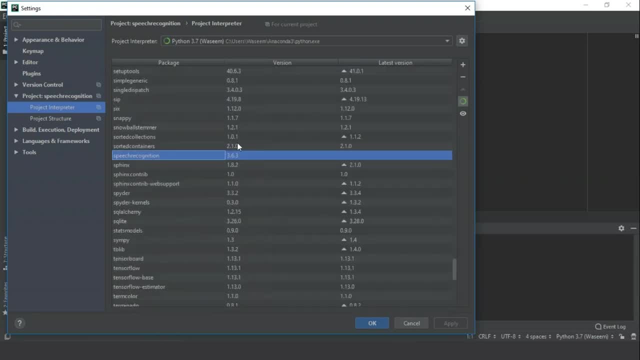 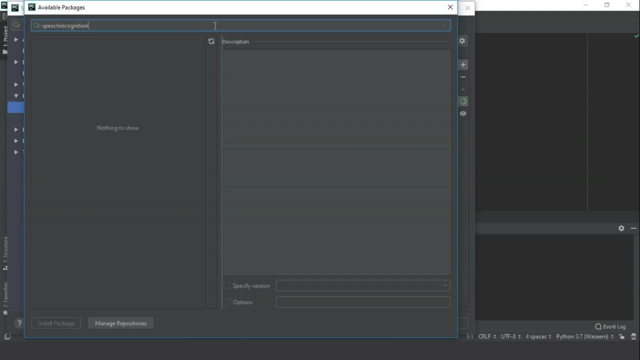 I'll show you where it is, as you can see, speech recognition already there, but you can add it. if you don't have it, You just type it over here, speech recognition, and you will find it and you can install it, guys. So this is as easy as it looks. 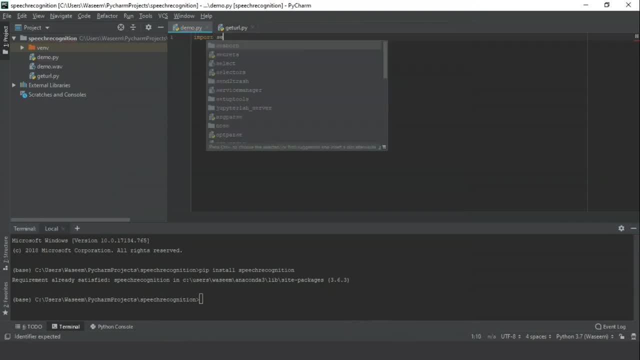 and to use it in your program. You can import speech recognition like this. You will find this package just imported as SR. Let's say so. we'll be using it, Using the speech recognition in our use case. So hang in there, guys. speech recognition has a recognizer class. 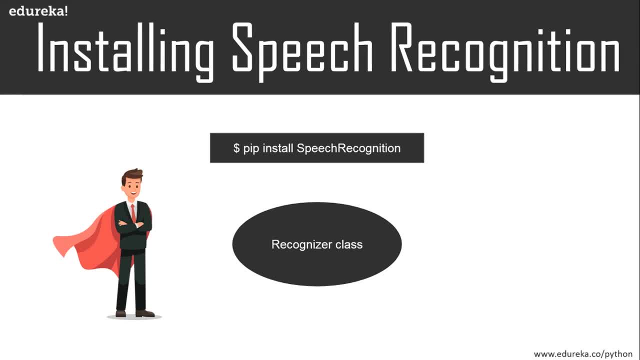 which is basically where the magic happens, or everything else that is connected to speech recognition is basically inside the recognizer class, So it has instances which are used to recognize the speech guys. So there are seven methods which can read various audio sources using the different apis. 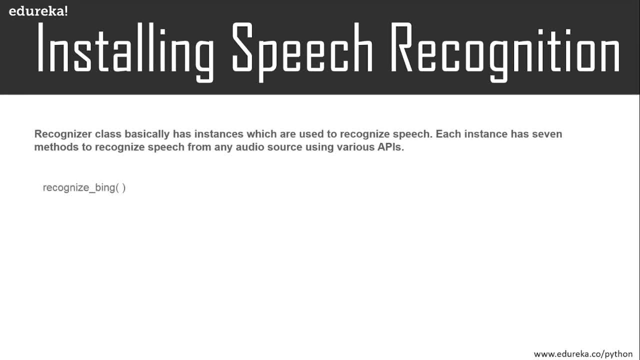 So let's take a look at those methods, guys. So first of all, we have recognized Bing, which is our Microsoft Bing search API, And then we have recognized Google, which is a Google web speech API, and then we have recognized Google Cloud, which is a Google Cloud speech. 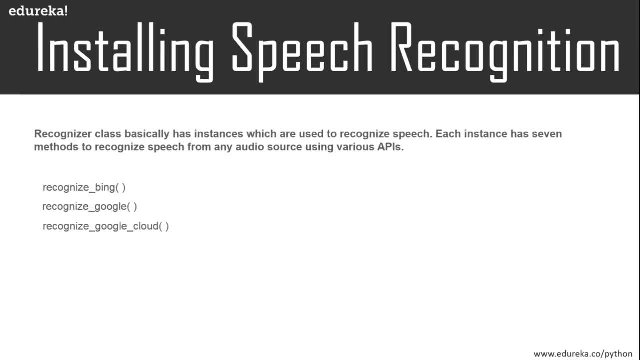 which also requires the installation of Google Cloud speech package. And then we have recognized hound if I, which was made by sound hound, and then we have recognized IBM, which was our IBM speech to text method guys. And then we have to recognize Sphinx. 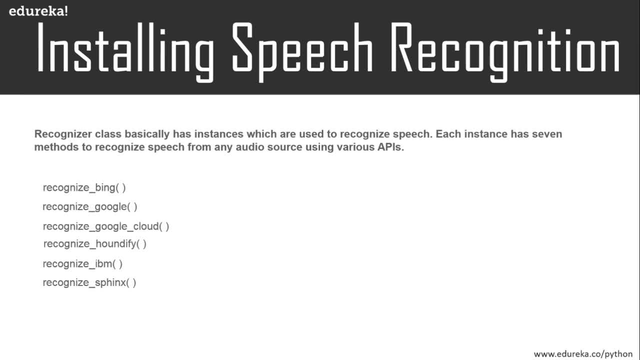 which is a CMU Sphinx module and which requires installation of pockets Sphinx as well, and it can also be used to run the speech recognition module offline as well. So if you want to run your module or if you want to run your program offline, you can use the recognize Sphinx method here. 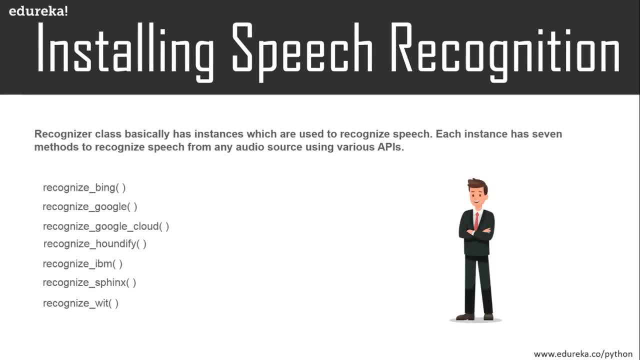 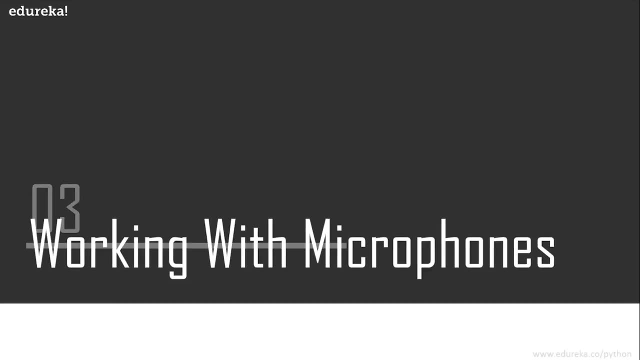 and then we have recognized wit as well, which is from wit AI package guys. So these are all the methods that you can use to record the audio from different sources using these apis. So now that we are done with speech recognition module guys, let's talk about how we are going to work with the microphones. 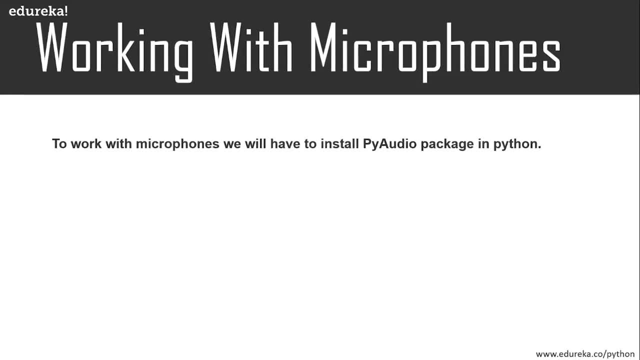 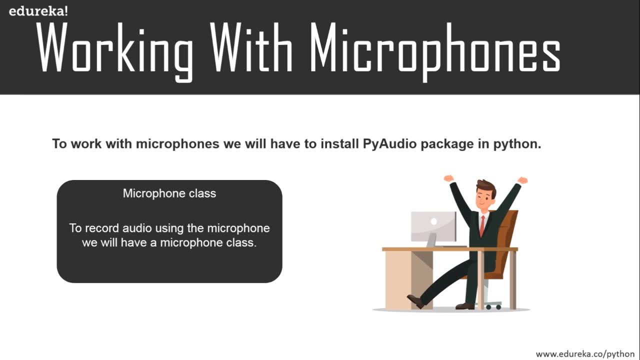 So to use the microphone we will have to install the pi audio module. So we will get back to this later. guys, Let's try to understand the microphone class, what it does and how we use it. So the microphone class is used to take the input. 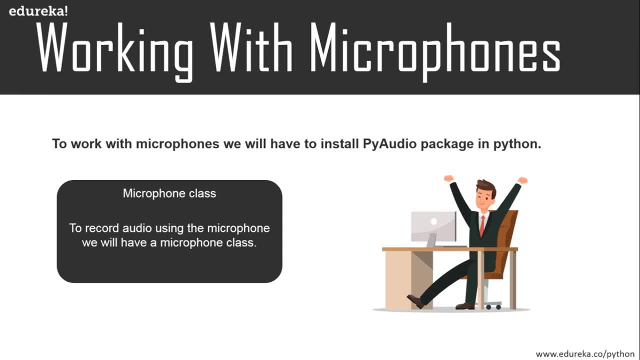 from the microphone instead of any audio file or any other source, guys. So we are using the microphone as the source, using the microphone class, for most of the projects. we can use the default microphones or, if you don't want to use the default microphone, 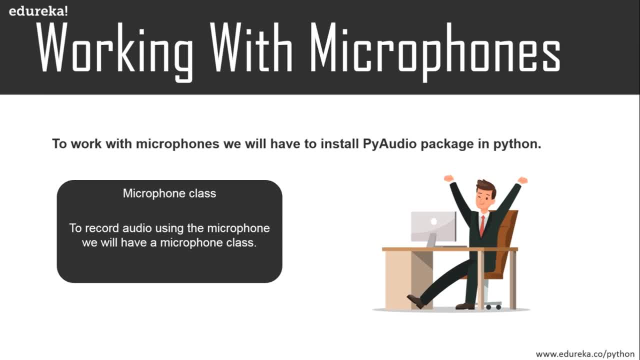 you can get the list of microphone names using the list microphone names method. now, to capture the input from the microphone, we use the listen method, So we'll be talking about that when we are working the use case guys, So you will be able to understand this better. 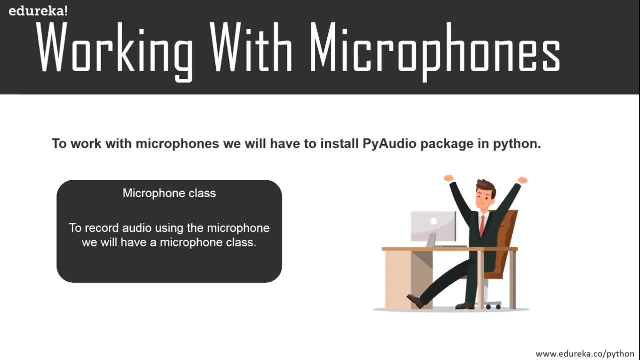 when we are working on the use case. So let's take a look at how we can install the pi audio module in python. So this goes without saying, guys: you will have to run the command pip install or pi audio inside your terminal. guys, 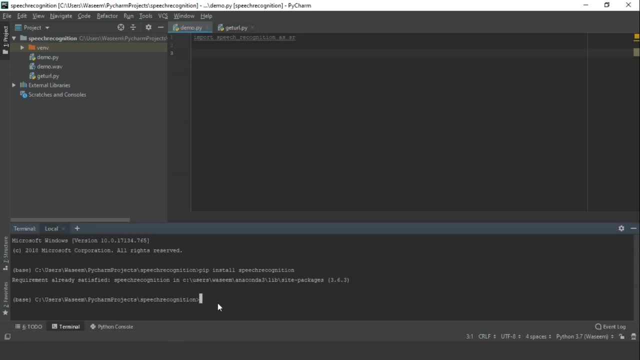 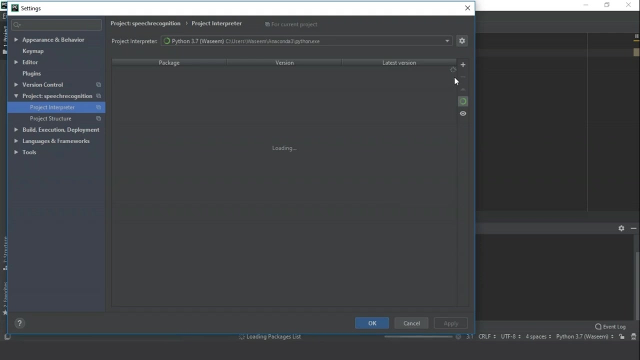 So let's take it up to pi charm again and over here in the terminal. I will just use pip install by audio, since I have already installed it. It's saying: requirement already satisfied and similarly you can install it using the project interpreter. guys over here. 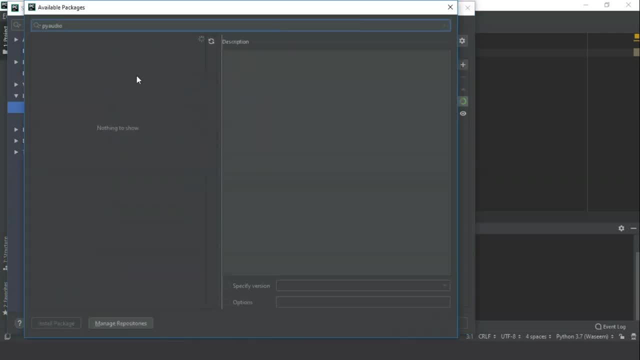 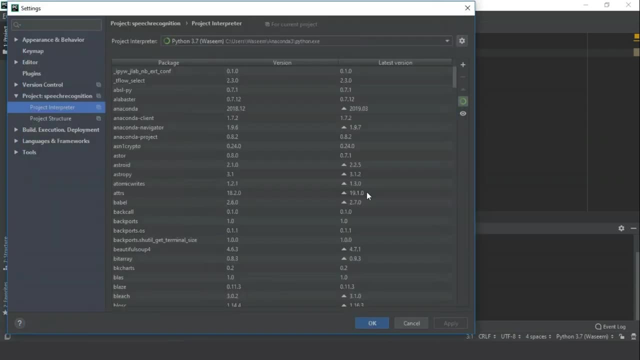 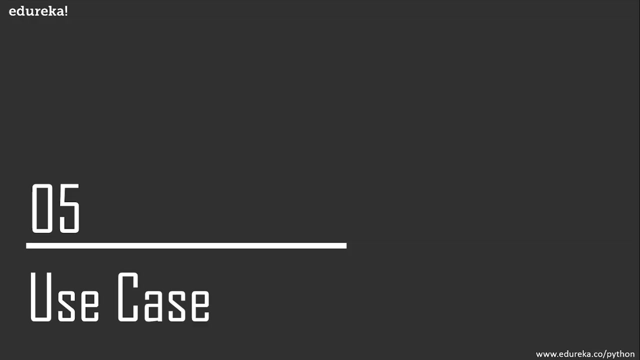 You can just type add, search pi audio over here. So there is this module and I can install it using this button over here, and it is as easy as it looks, guys. So now that we have installed the pi audio module as well. So let's talk about the use case now. 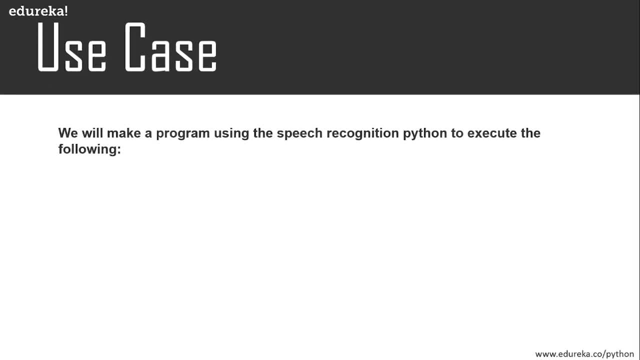 So we have a problem statement in which I'm going to make a program using the speech recognition python module to execute the following. So, first of all, I'll be converting the speech to text using the speech recognition module and then using the text to open a URL using the web driver. 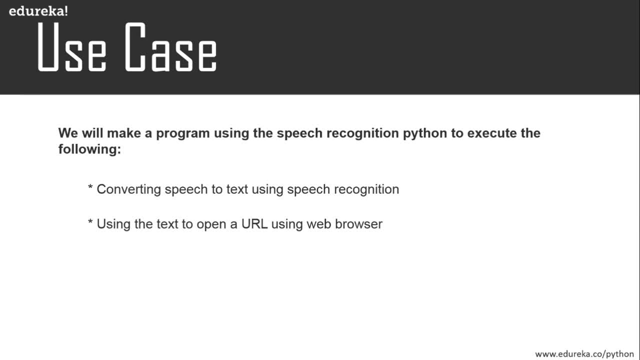 So, guys, I'll be using one more module, which is web driver, to actually use the text that I'm getting from the speech recognition module to open a URL and inside the URL also will be trying to search a query using the speech recognition. So let's take it up to pi charm, guys. 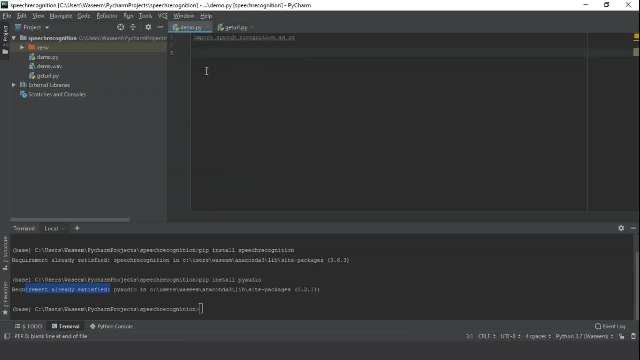 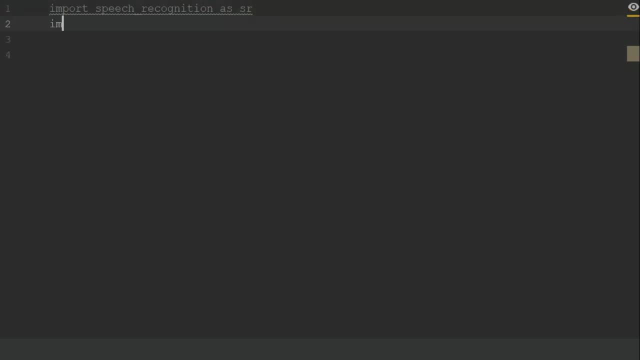 and we'll try to make a program using the speech recognition module. So let's take it up to the presentation mode, guys. So I've already imported this speech recognition module. I'll import web driver as well. I'm sorry, web browser guys. 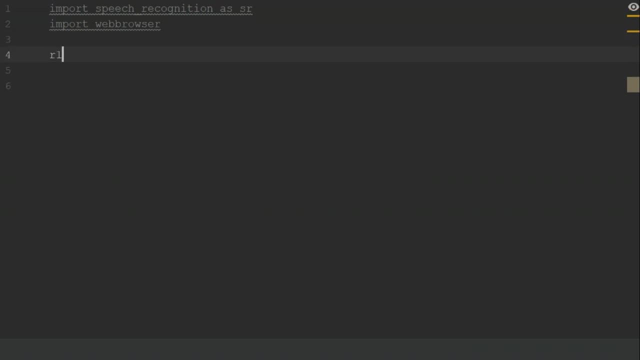 So what I'll do is I'll make instances now. So I'll just make our one is equal to SR dot, the recognizer class that I was talking about, guys. So we'll make three instances, because we are going to need three instances here. So we'll make one more recognizer class. 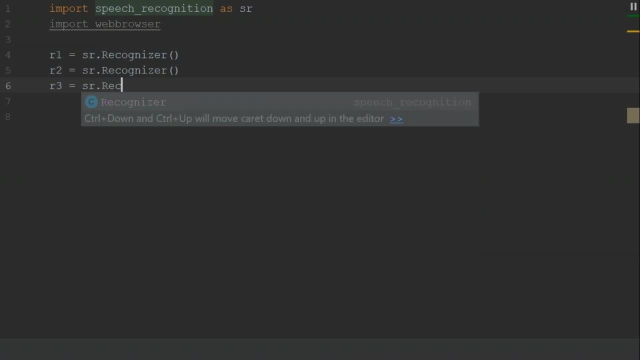 And our three is equal to SR dot. So we have made these instances which are going to take the input from. so we have to specify where the input is coming from. So I'll just write with SR dot microphone As source, because this is going to be our source, guys. 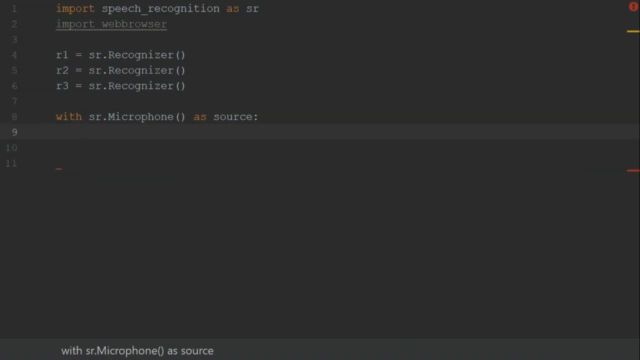 so you don't have to worry about where the source is coming from. So what I'll do it. I'll just print a statement. Let's say I want search query as what all links I'm going to provide guys, So I'll be actually using two URLs. 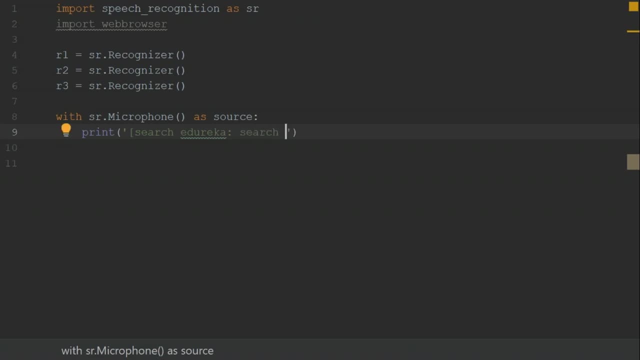 First one will be the URL to our edurecoco page, And then the next one will be the YouTube URL, guys, and then I will write: speak now. So what I'll do is I'll take one variable, Let's say audio, and in this I will actually use the instance. 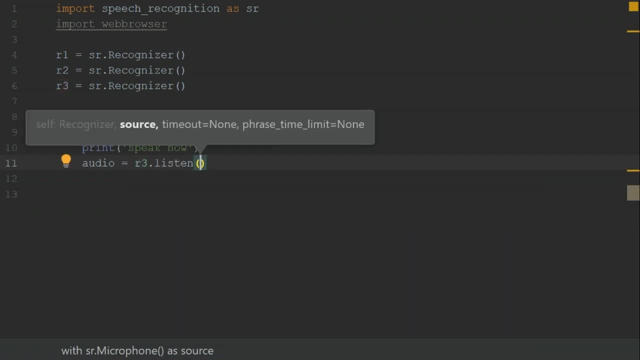 and you will use the listen method Now. So listen method is going to take our input from the source, which is actually our microphone. guys. Now, what I'll do is I'll make the queries, guys. So if the query is actually, let's say, edureco, 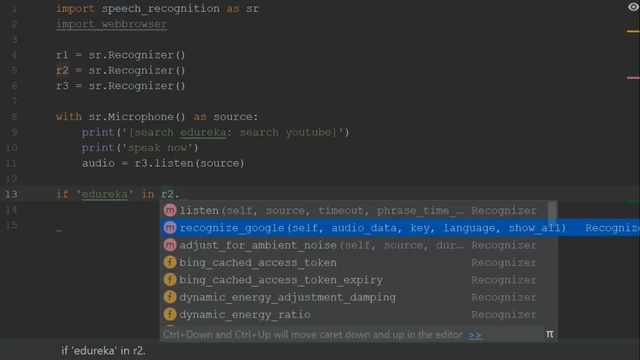 So now comes the API that I was talking about, the seven methods that I showed you. so I'll be using this recognize Google guys. Similarly, We have recognized being in all those things, So we'll just be using recognize Google here and inside the recognize Google. I will pass the audio. 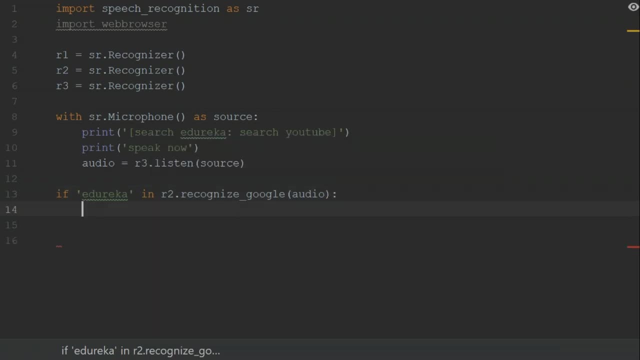 It will actually translate the audio into the text, guys. So this is why we use recognize Google over here. So what happens is I'll use the instance now. So we have one more recognizer are two that we have already specified over there. Now, what I'll do is I'll pass the URL, guys. 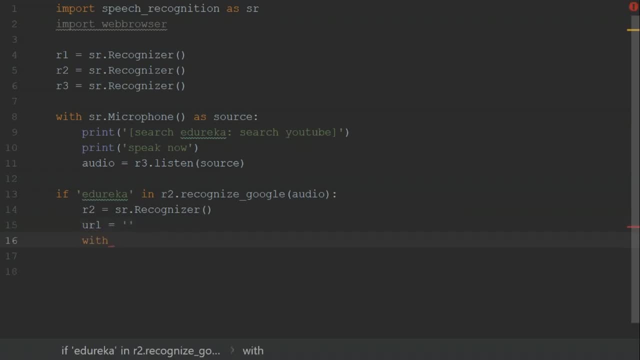 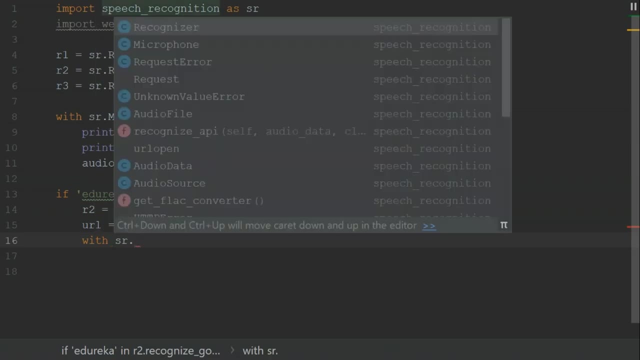 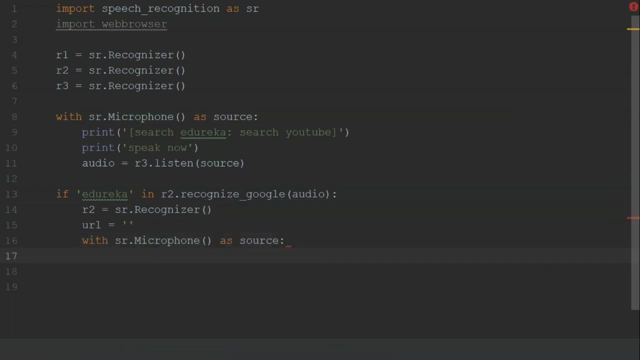 So inside this I will paste the URL later, guys. So we need another input, guys, because we are going to search as query as well inside the URL. So what I'll do is I'll take microphone again as source. Now what happens is I will print, let's say, search your query. 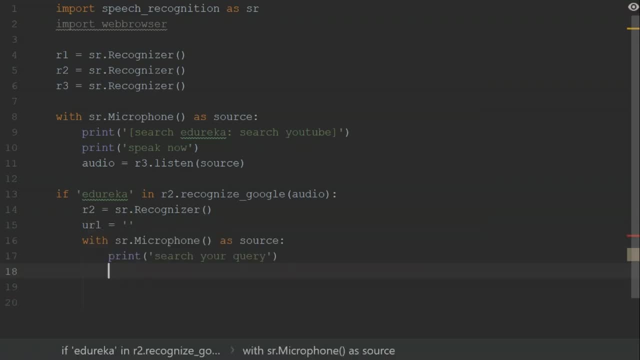 Now what happens is I will have one variable, Let's say audio, and then inside this I will pass the instance and I will use the listen method again and pass source into this. Now I'll have to make a few changes, guys, So for this I will make one try statement. 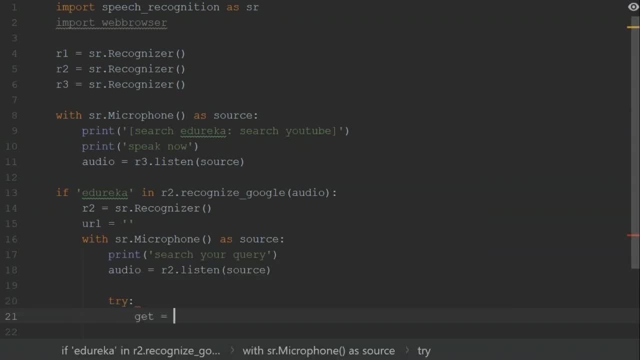 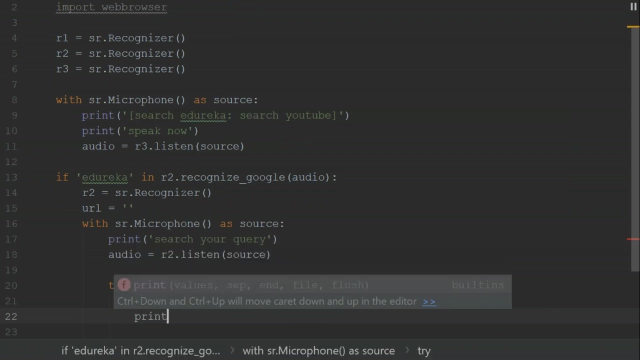 and inside this I will pass a variable, Let's say get, and inside this I will pass one more instance and we will recognize Google API using this as audio. So this will recognize our input. the second query, that is. so we'll print get now. 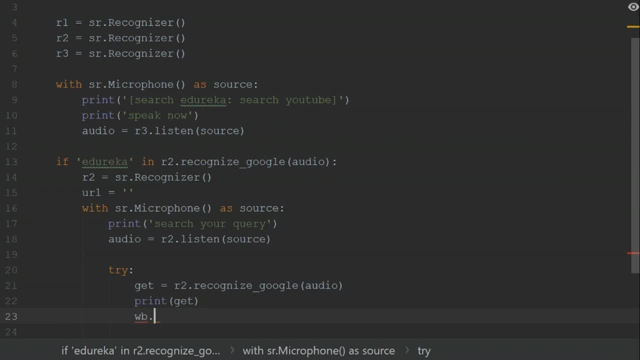 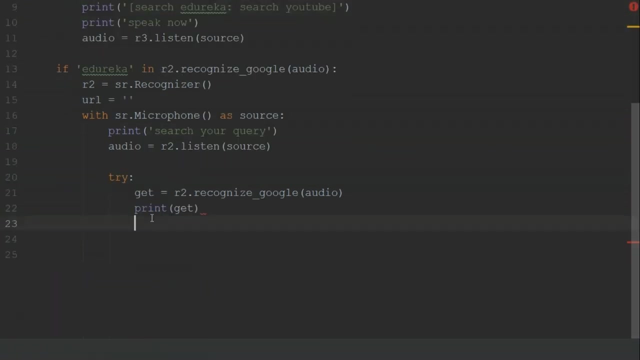 And we will also use the web browser module that we have specified guys to get or to open a new. Okay, Okay, one second right. I have not given it any alias. I'll give it as WB. now I'll write again: WB dot get and open new. 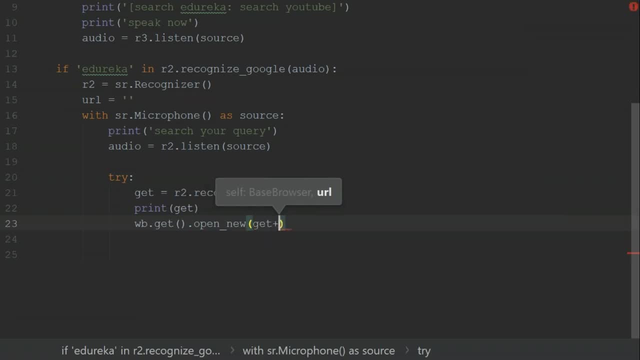 and inside this I will pass get and the URL. guys, I'll pass URL first and after that get, so this will actually open our URL using the URL that will I will specify over here, and after that I will get Get the query using the speech recognition. 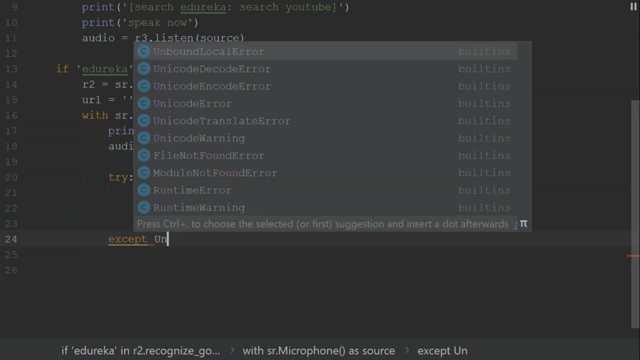 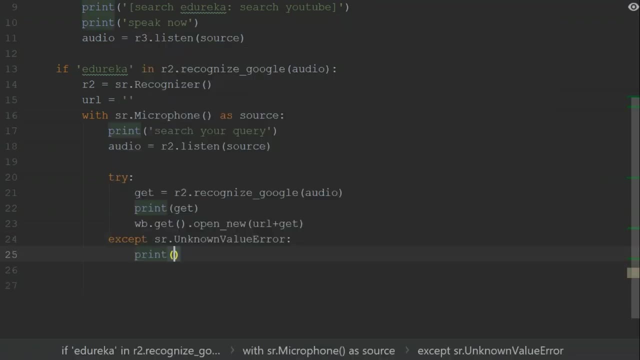 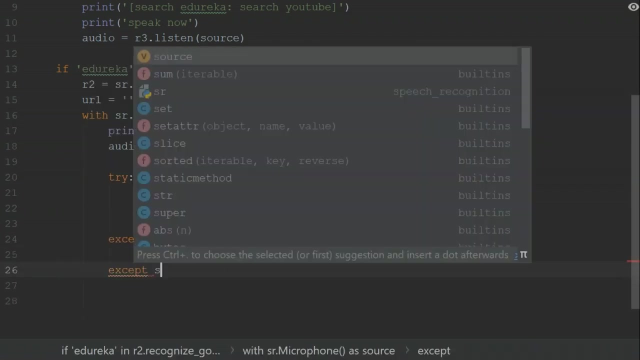 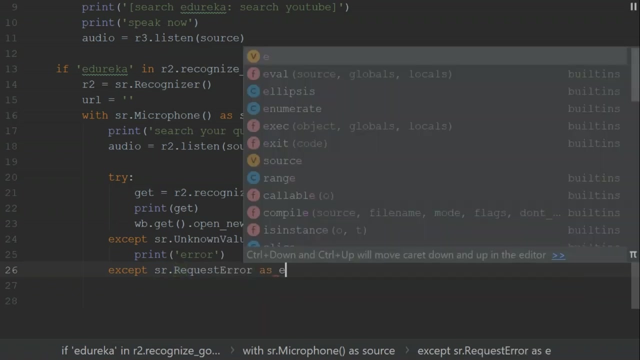 Now I'll pass some exceptions, guys. So I'll pass unknown value error. Okay, SR dot- unknown value error. I will print error. Now I'll pass one more exception, guys, and inside this I will pass SR dot- request error. Let's say as E, and I will print. 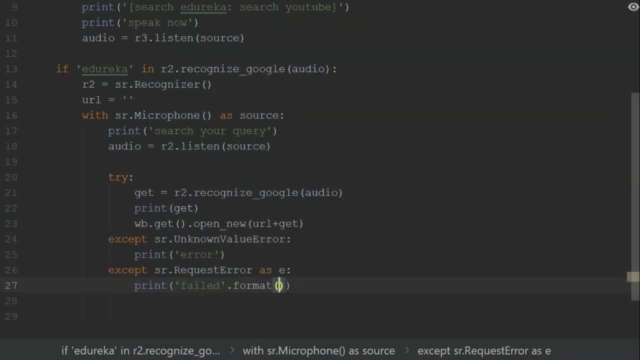 error, or, let's say, failed dot format of this E. now let me run this, guys. Okay, we will have to use the URL as well. So what we'll do is we'll paste the URL over here. Now let's run this, guys. 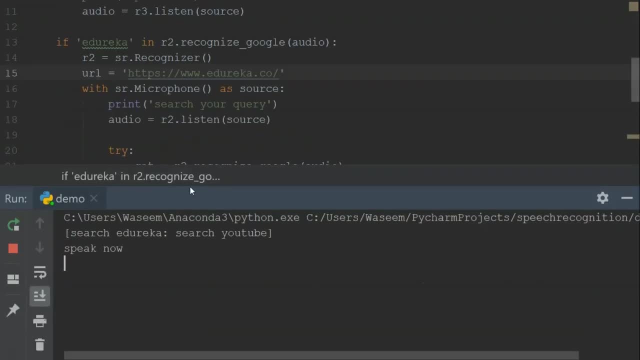 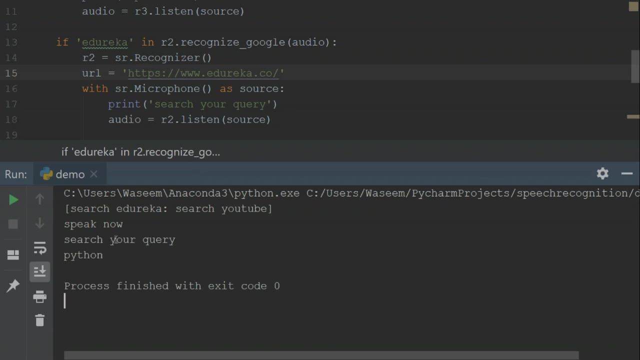 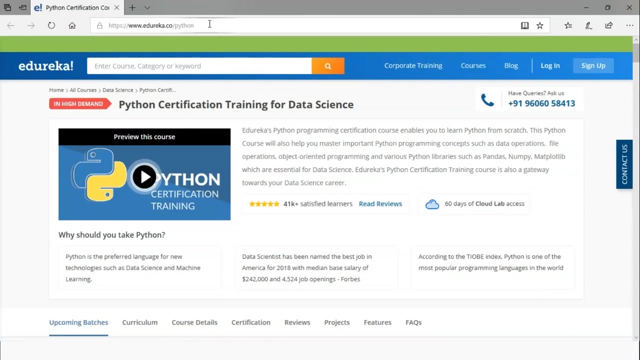 You will see how it's working. So now, when I say edureka Python, now you must be wondering. there is nothing happening. I'm just getting the speech from the text, but in the background, we have already got this web page open using our speech recognition model for this. 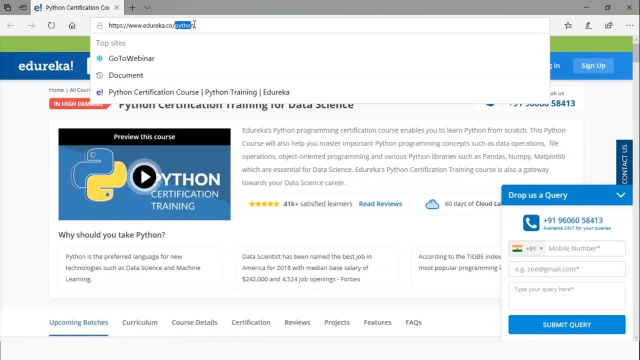 This is the URL I had provided and this is the query that I'm getting from the speech recognition model. So, as you can see, guys, this is what you can do using the speech recognition model. Now let's take it up to PyCharm. 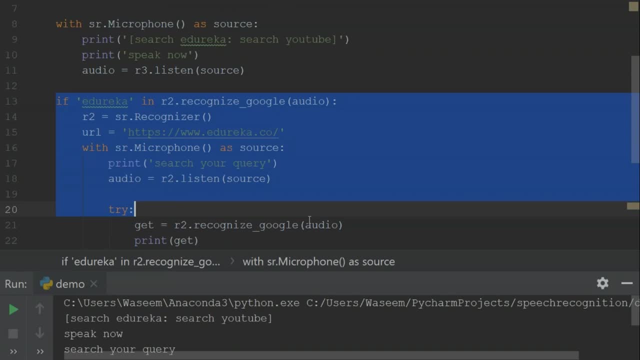 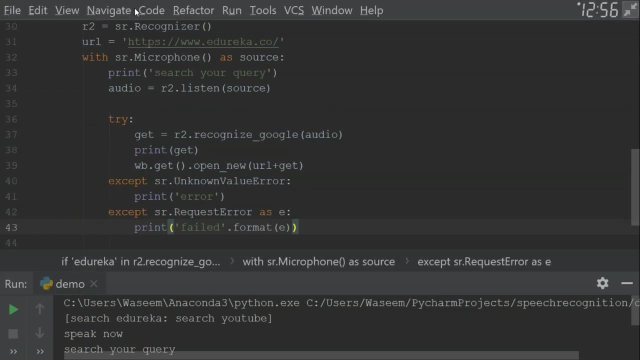 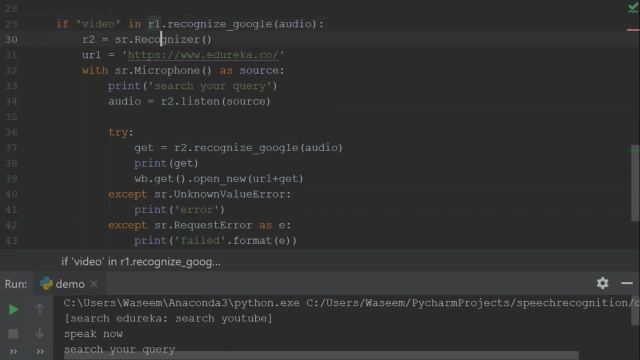 and so we'll give it one more query to work. So instead of edureka, let's say I want video as well. So just copy the same thing and instead of edureka I'll write. let's say video, and instead of r2 I'll replace it with r1. 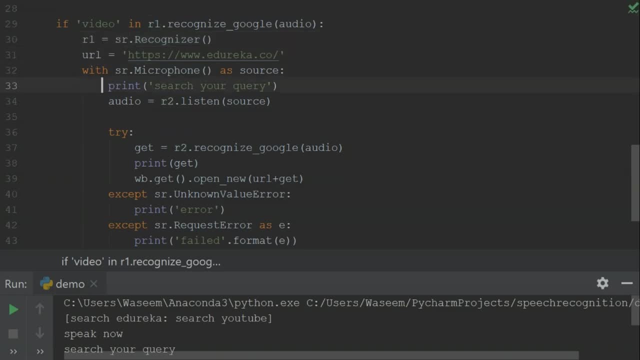 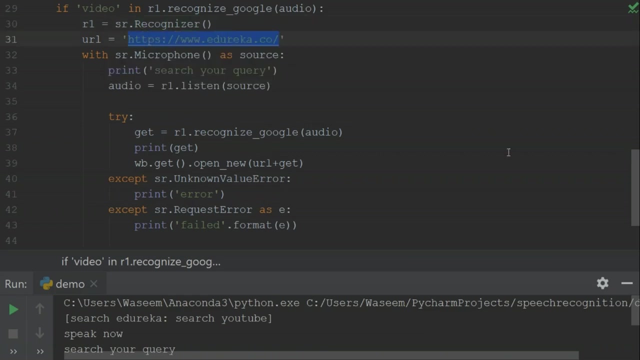 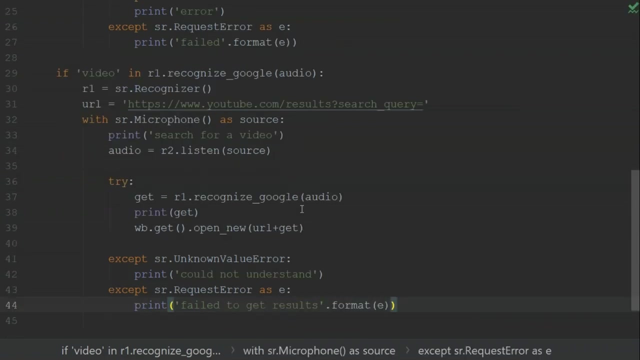 because we have different instances for these. I think everything is correct. We just have to replace the URL, guys. So I'll copy the URL now. So I'll replace this URL with the URL that I want, which is the YouTube one, Now that we have replaced the URL as well. 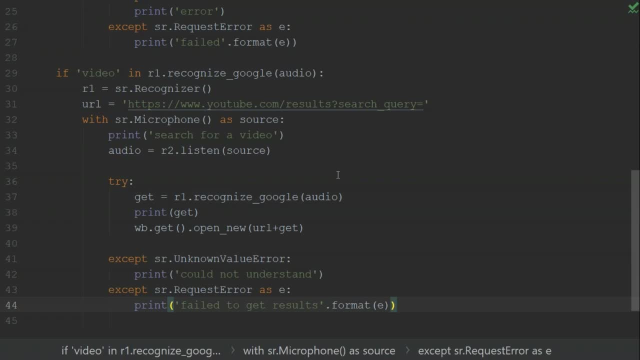 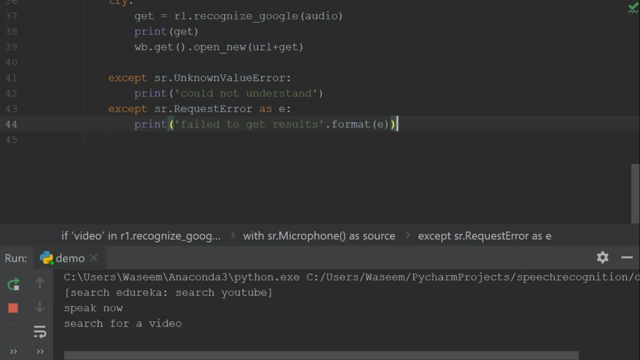 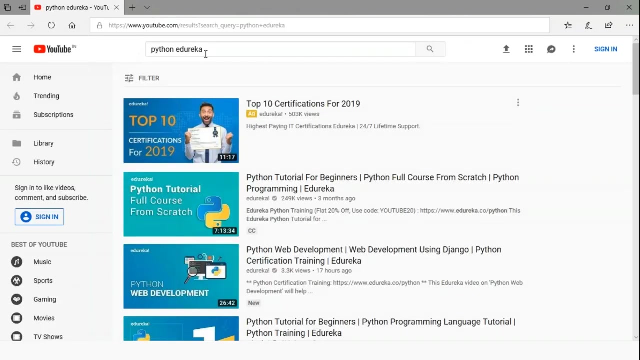 Let's run this now. So instead of edureka, I will just say: okay, let it load Video Python, edureka. So, as you can see, guys, I have opened this URL and I have also entered the query string, guys, using the speech recognition. 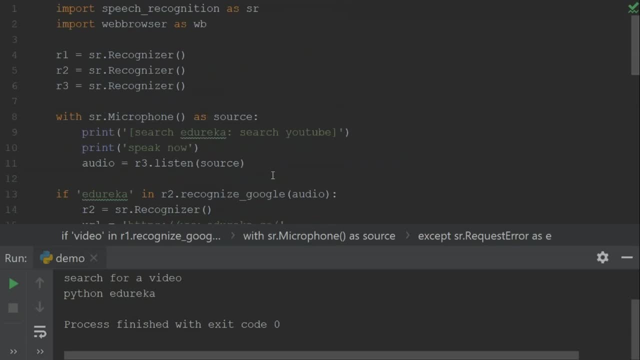 So to get a clear understanding, I will show you once again what I have done in the program. So I have imported The speech recognition module and then I have imported the web browser as well. Then we have made three instances: r1, r2 and r3.. 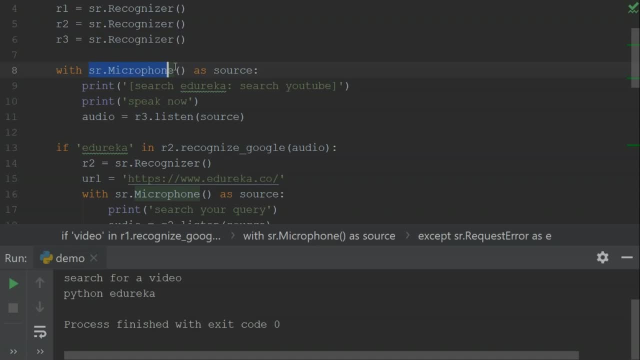 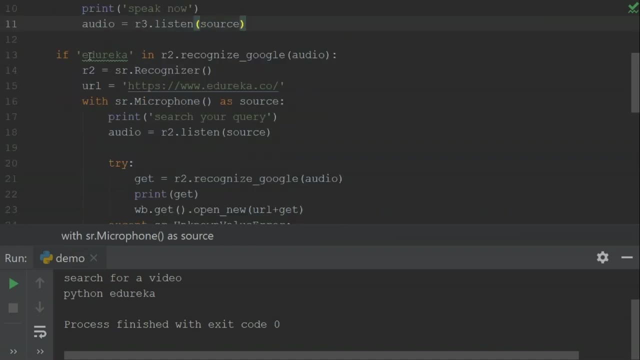 So these are the instances that we have made, and after that we have specified the microphone as source in which we are getting the audio using the listen method here and after that we have different queries that we want to search. So if I say edureka and it recognizes as edureka, the text will use. 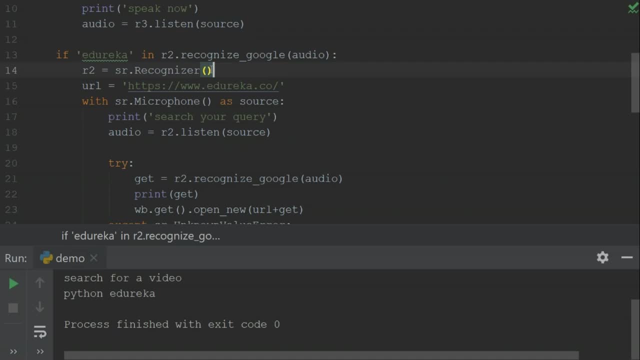 the recognize Google module again and it will take one more instance, that is r2, and it will take This URL and we will get the source as microphone and put the query as speech and that query will be added to the URL and that is how we are going to execute this command. 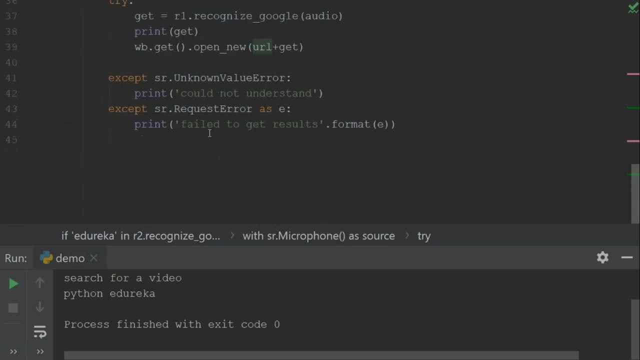 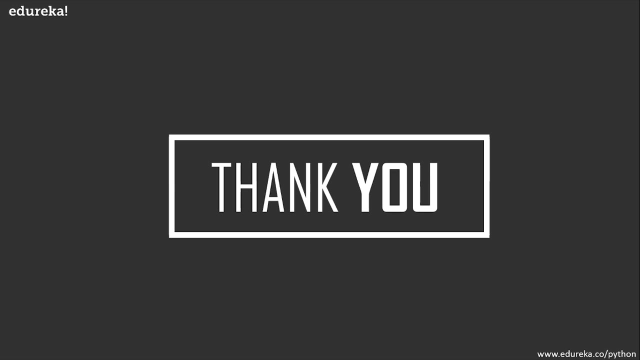 and similarly, for if I am saying video will be using that same as well. So now that we have come to the end of the session, guys, I hope you are clear with the concept of speech recognition module in Python And if you have any questions. 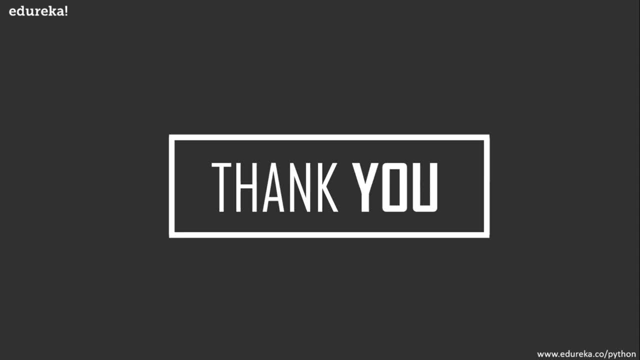 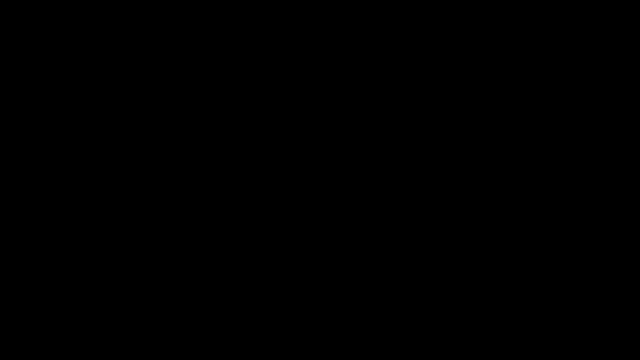